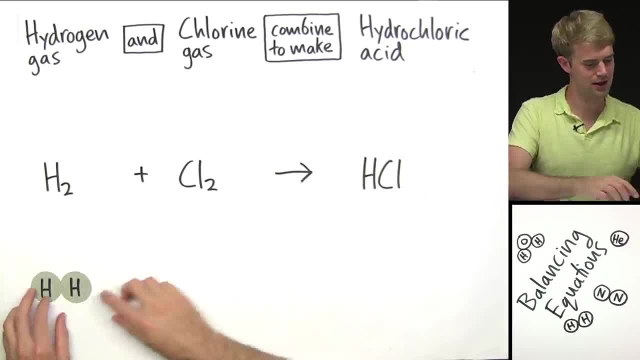 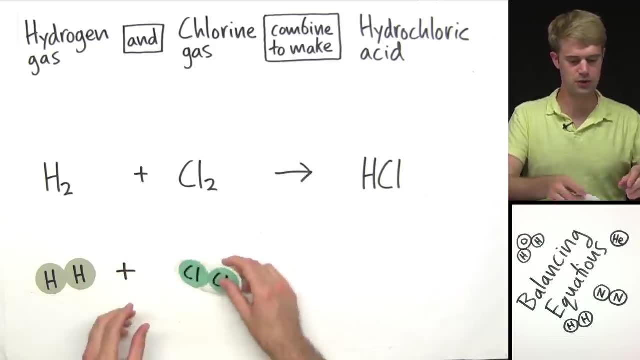 Okay, so we've got a molecule of hydrogen gas. It looks like this: We've got two hydrogen atoms, 1, 2.. Then we've got some chlorine gas. We've got a molecule of that 2 chlorine atoms. We've got our arrow. 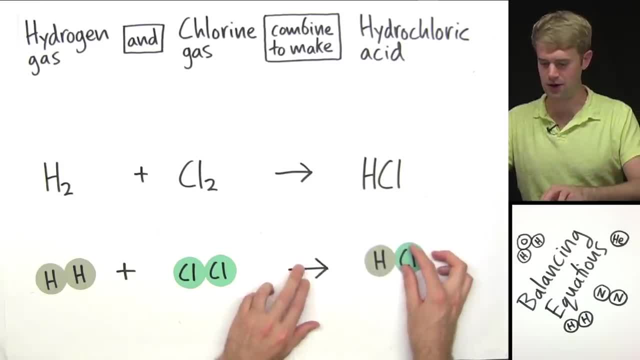 finally, a molecule of hydrochloric acid. So there it is: one hydrogen and one chlorine. Okay, so now we're going to start talking about balancing equations and balanced equations. First thing that I want to do is figure out whether this equation here is a balanced equation. 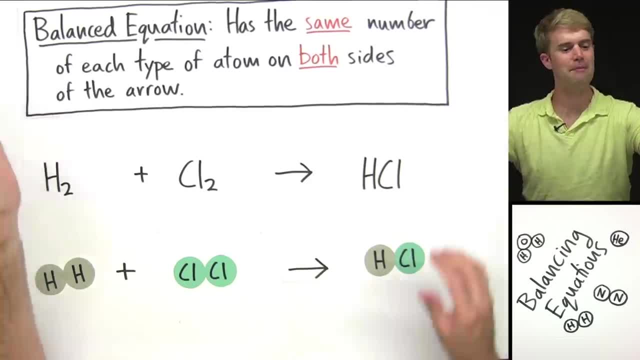 So here's the definition for balanced equations. A balanced equation has the same number of each type of atom on both sides of the arrow. Okay, so, keeping this definition in mind, what I have right here, is this a balanced equation? No, it's not. Here's why. On this, 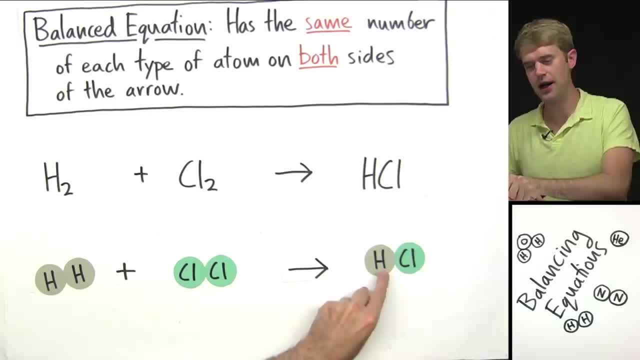 side of the arrow I have two hydrogen atoms, over on this side I only have one. Over here I have two chlorines and over here I only have one. So this is not a balanced equation. We don't have the same number of each type of atom on both sides. 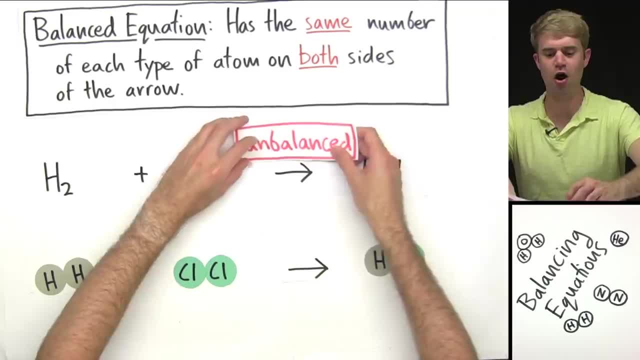 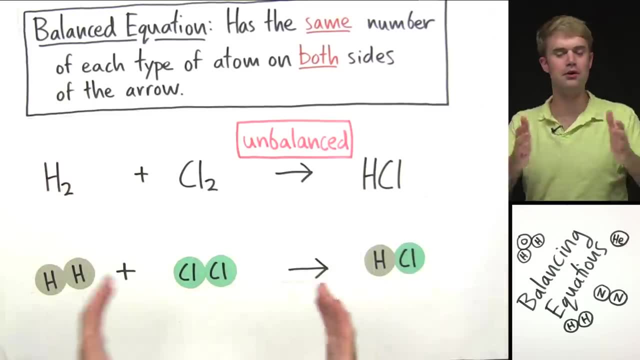 This isn't a balanced equation, so we call it an unbalanced equation. Unbalanced is just the word for an equation that's not balanced. It has different numbers of one or more of the types of atoms on the two sides of the arrow. Okay, so this is currently an unbalanced. 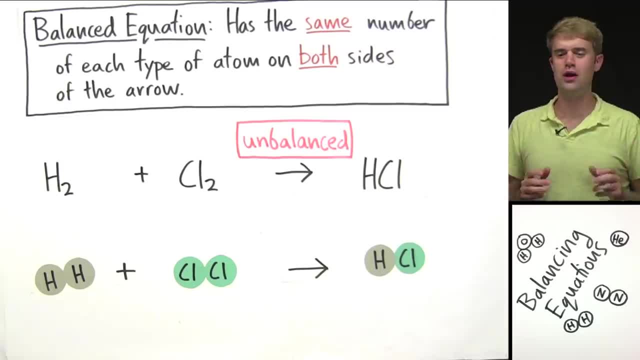 equation. Now, most of the time in chemistry unbalanced equations aren't particularly useful to us and we have to make them balanced before we can use them for problem solving or for doing calculations. So often in chemistry we start out with unbalanced equations and 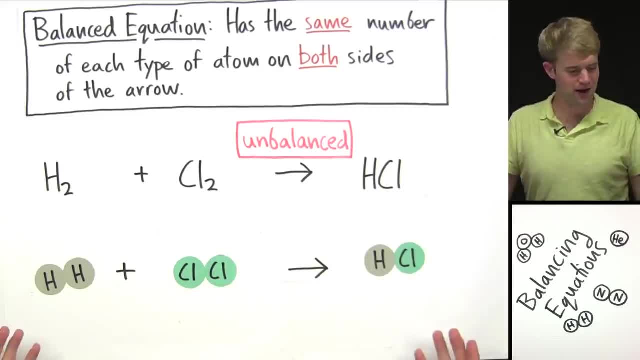 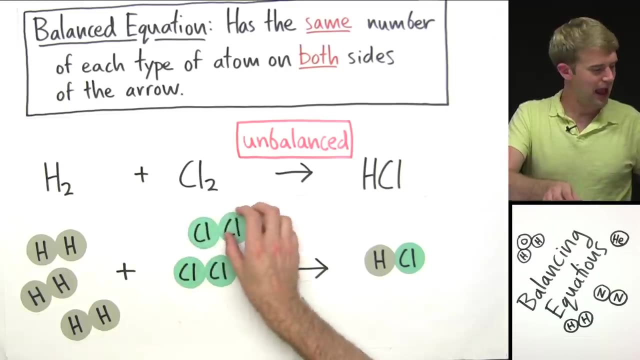 then we have to figure out how to balance them. So, in order to balance this, we're going to make a few adjustments. Here's how we do it: To balance the chemical equation, we change the number of these molecules that we have and we find a combination that gives us the 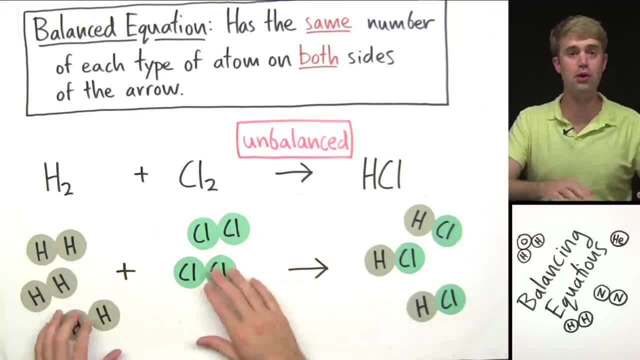 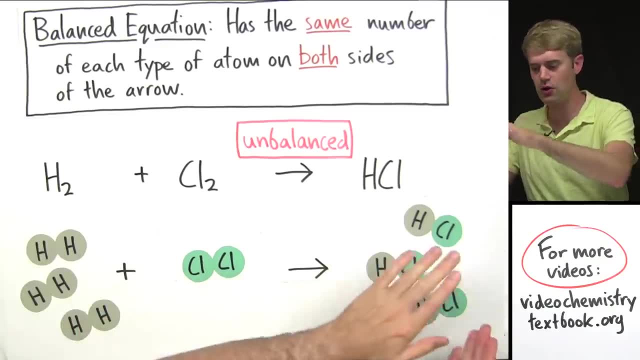 same number of each type of atom on both sides. Okay, it's a little bit like a puzzle. So it might turn out that to balance this equation, we need three of these and one of these and three of these, Or we might need two of. 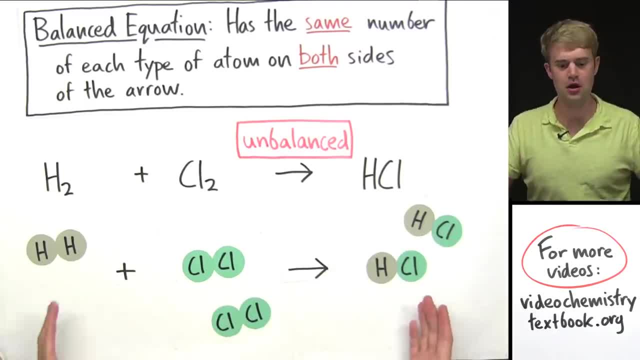 these, and two of these and one of these. So we play around with the number of each one of these that we have, finding a combination that gives us the same number of each type of atom on both sides. Okay, so take a look at this equation. Can you figure out what? 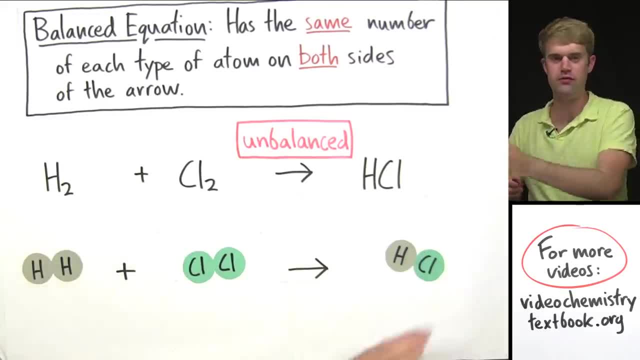 we need to do to one or more of these in order to have the same number of each type of atom on both sides. Well, here's what we do. We have two hydrogens here, two chlorines here: one hydrogen, one chlorine. So if I get another one of these, okay, if I have two of these. 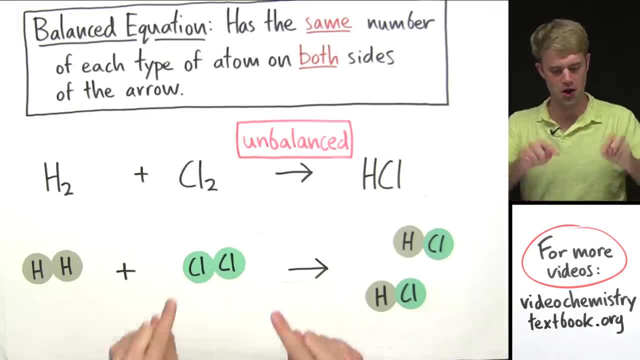 we'll then have two hydrogens here, two hydrogens on this side, two chlorines on this side, two chlorines on this side, And now this equation is balanced. Okay, so we've balanced the visual, the visual version of it To balance. 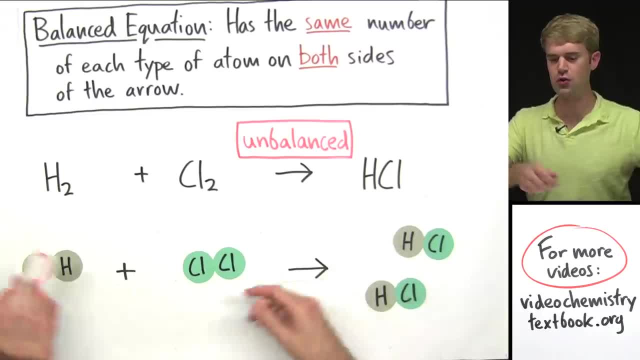 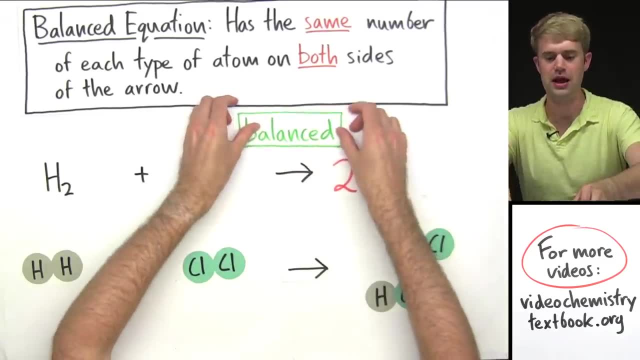 the written equation. what we'll do is we'll put a two in front of the HCl here to show that we have two of these, And now the equation is balanced. Okay, so this is the combination. this is the combination of these things and these. 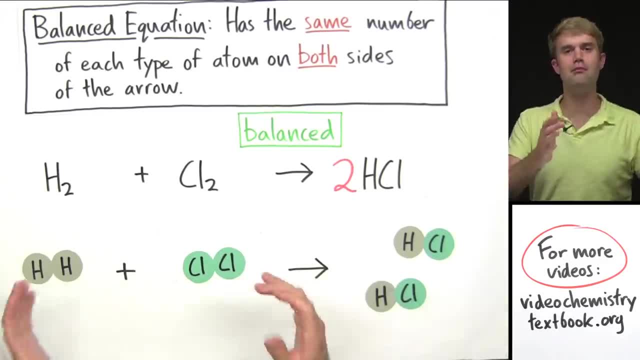 things that we need to have the same number of each type of atom on both sides. We need one of these, one of these and two of these to end up with a balanced equation. Here's another chemical reaction: Hydrogen gas and oxygen gas combine to make water. 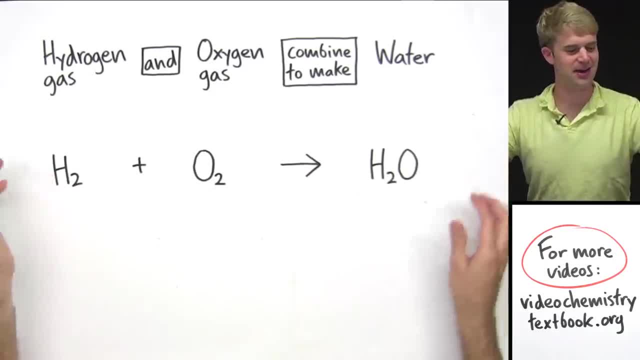 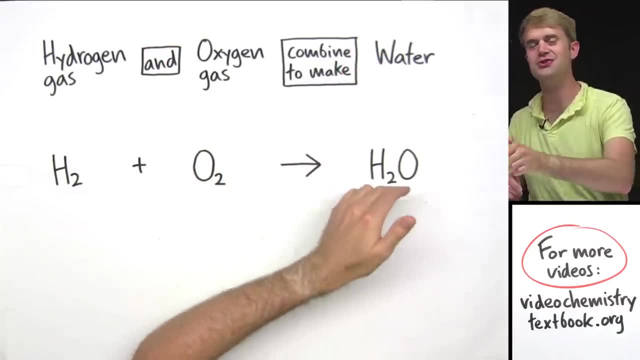 The chemical equation for this looks like this: The chemical formula for hydrogen gas is H2,, then oxygen gas is O2, and these combine to make water, which is H2O. Now let's look at how we can represent this visually. Okay, we've got one molecule of. 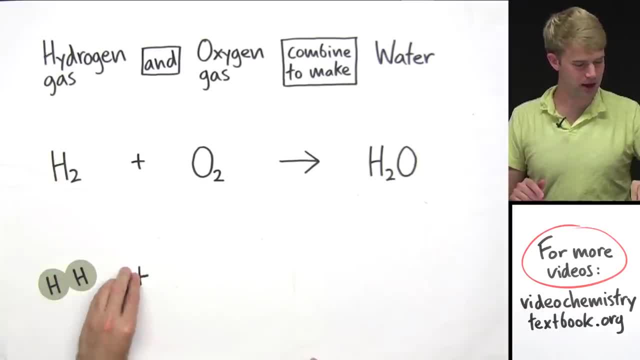 hydrogen gas, H2, then we have one molecule of oxygen, gas O2.. We've got our arrow here and H2O water is over here. Okay, so, just like we saw previously on this side of the equation is what we start. 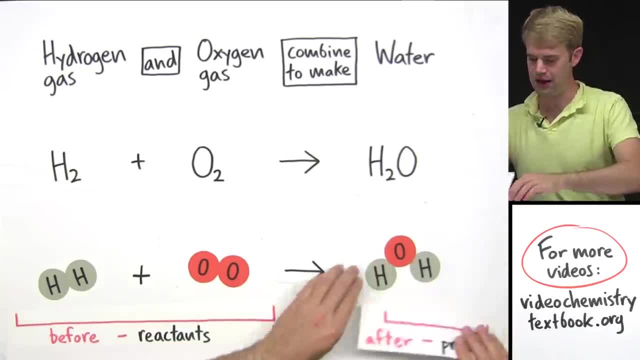 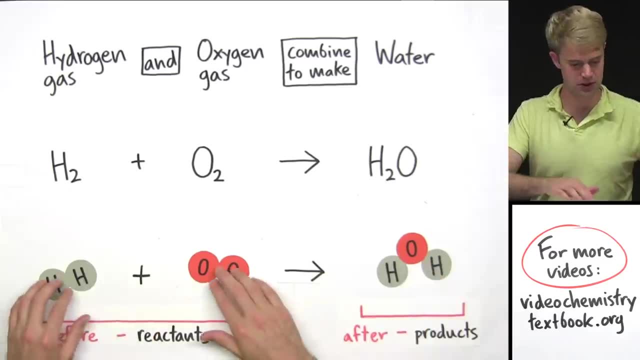 with. It's our before we've got our reactants, and over here is our after our products. Okay, so take a look at this equation and these atoms here and think about this. Is this equation balanced the way it's written here? 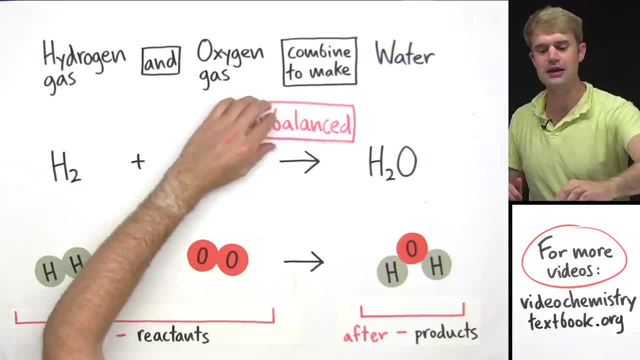 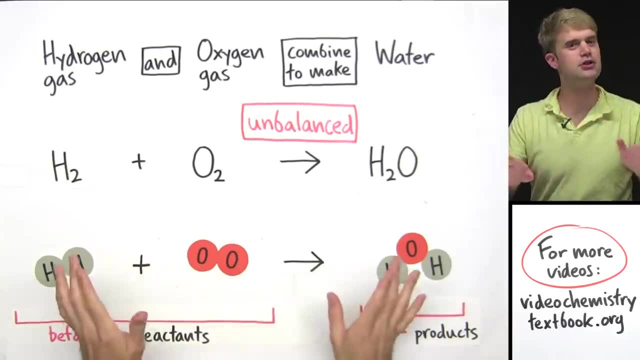 And the answer is no, It is unbalanced. Here's why I've got two hydrogens here and two hydrogens here, So the hydrogens do balance, but the oxygens don't. I have two oxygens here and only one over here, so this equation is not balanced as it's written. 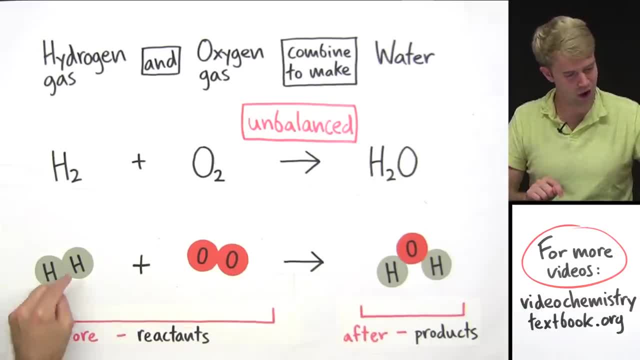 In order to change this, we're going to adjust one or more of the numbers of these different compounds. Okay, here's how we're going to do it. Take a look, I've got two oxygens here and one here, So the first thing I want to do is I want to try to balance these oxygens. 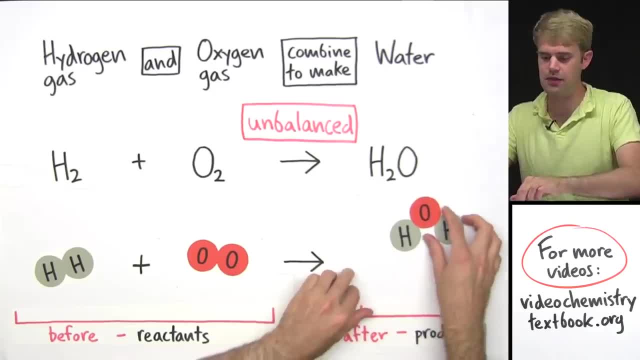 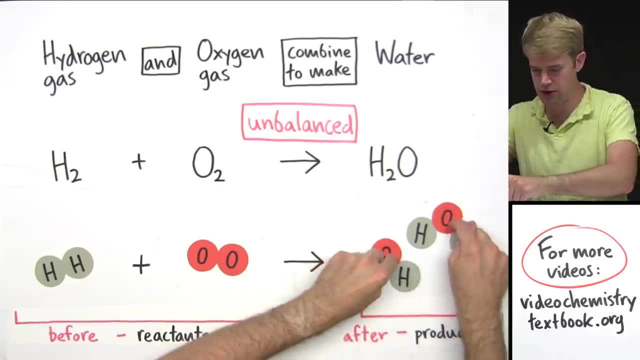 To get more oxygens on this side, to get two oxygens on this side, I'm going to add another one of these H2Os, So now I have two of them. All right, so I have two oxygens here, two. 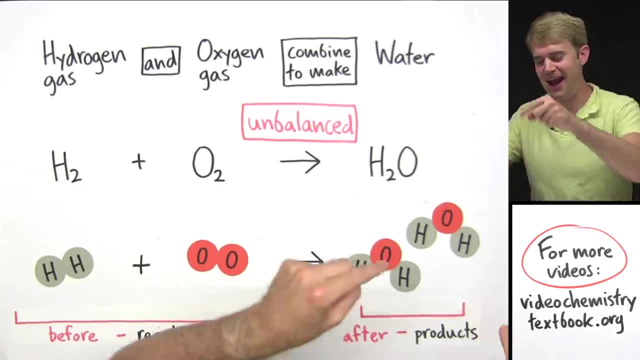 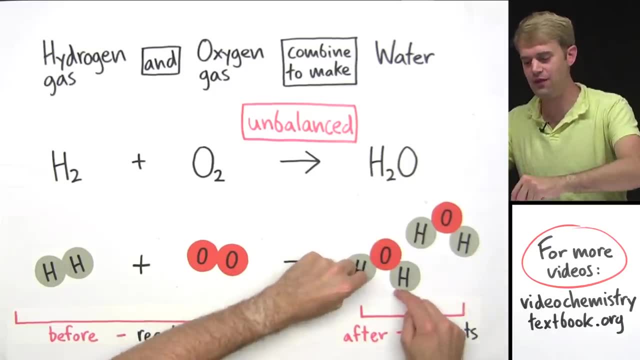 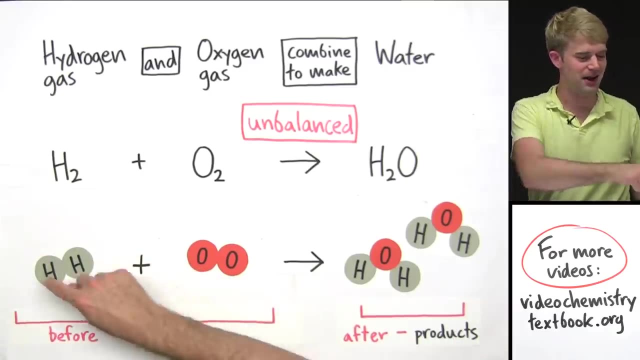 oxygens. here The oxygens balance. But check this out: By adding this water here, I change something else. My hydrogens used to balance, but now I have four on this side. I only have two on this side, And that's okay, because I can change the number of these as well. Okay, I used to have one. 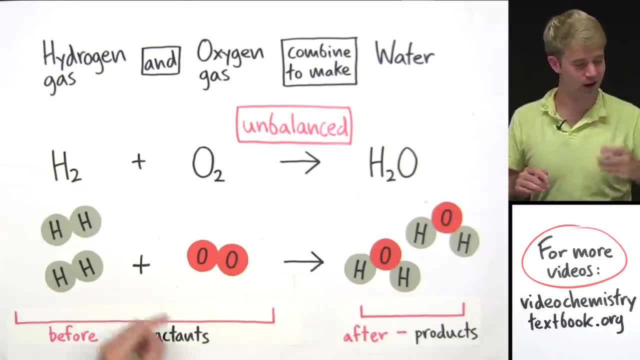 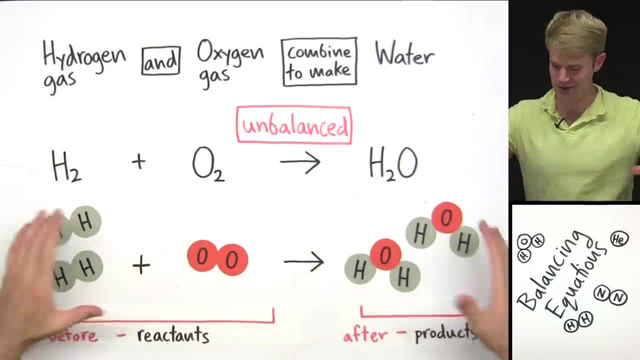 so let me add another hydrogen here. Now I have four, One, two, three, four hydrogen atoms over here and one, two, three, four hydrogen atoms over here. Okay, so now this is a representation of how the atoms balance In order to balance the chemical equation. 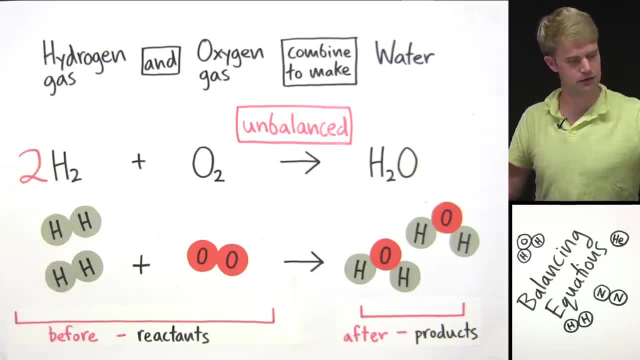 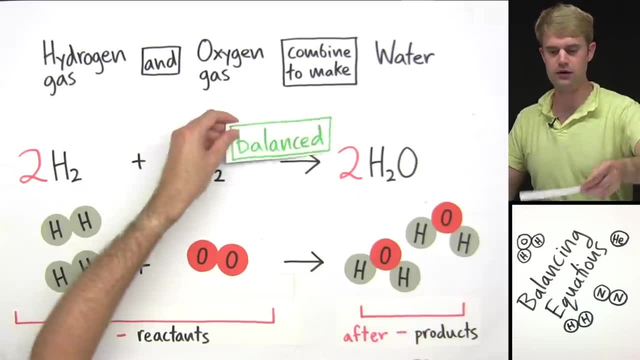 up here. I'm going to put a two in front of the H2, because I have two of those, and then I'm going to put a two in front of the H2O Here, because I have two H2Os, and now the equation is balanced. Here's a really common 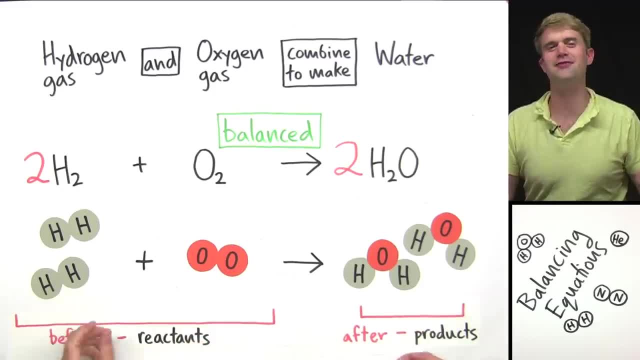 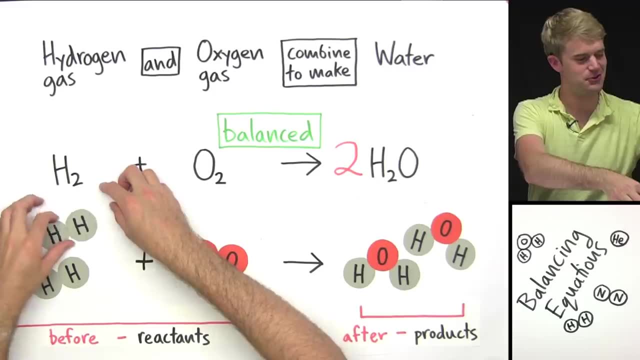 mistake I've got to tell you about When people are first learning this stuff. a lot of the times they'll say, hey, I have a simpler way to balance this. Here's how you do it: Get rid of this two here, get rid of this two here, and then just put a little number two. 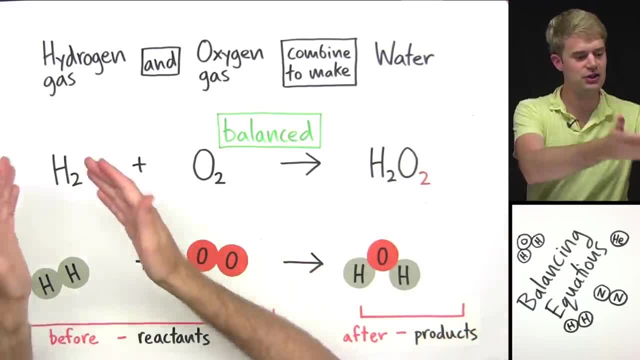 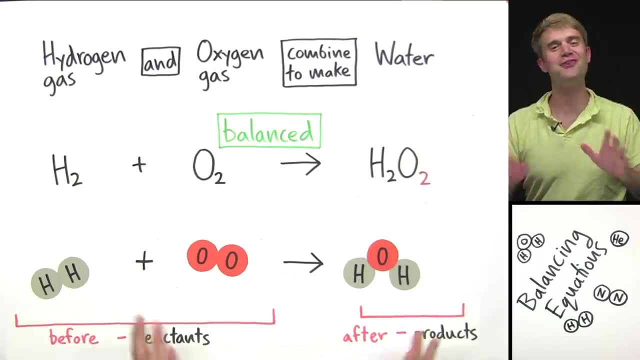 right under this O here. Now you have H2 on this side, H2 on this side, O here, and then O2 on this side and O2 on this side. It balances perfectly. Yeah, but unfortunately you can't do that. These numbers here, we call them subscripts, You can't change them. 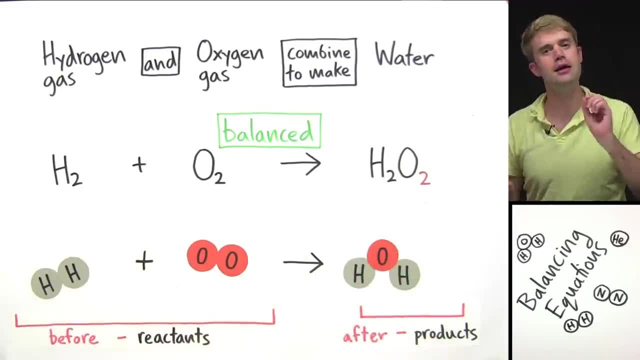 when you're balancing an equation, They have to stay the same, and here's why, In this equation, we're talking about water. Its formula is H2O, and this is what a water molecule looks like If you put a two here. we're not talking about water anymore. We're not talking. 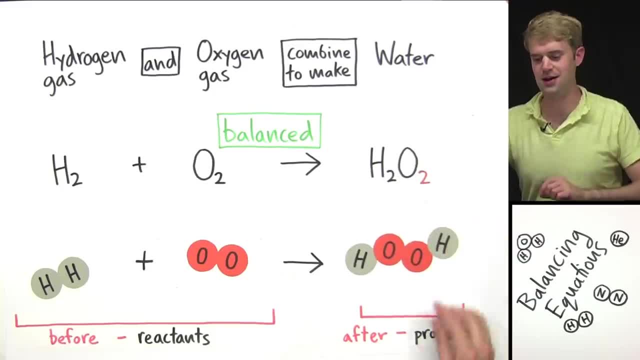 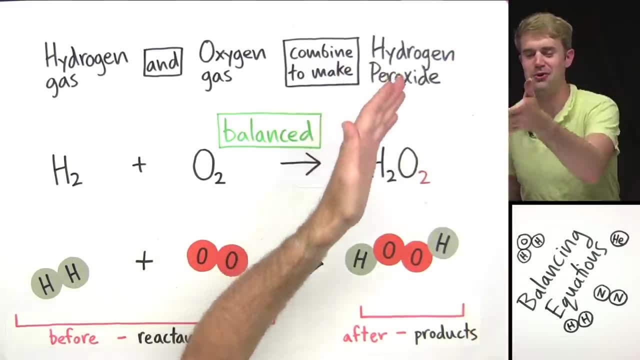 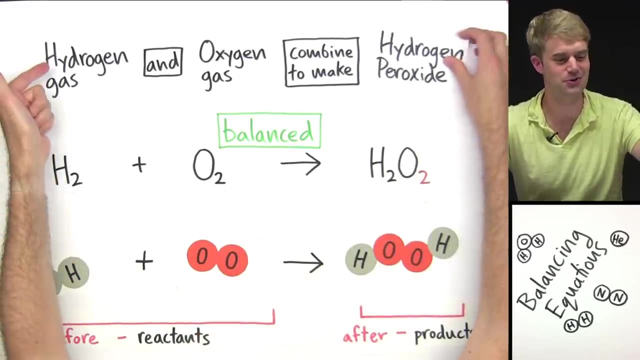 about H2O anymore. We're talking about a molecule like this with two oxygens and two hydrogens. This isn't water. This is now a compound called hydrogen peroxide. So yeah, by adding this two you might balance the equation, but it's no longer the equation for hydrogen gas and oxygen gas. 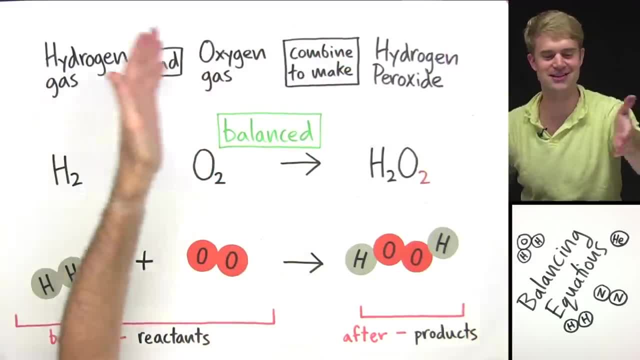 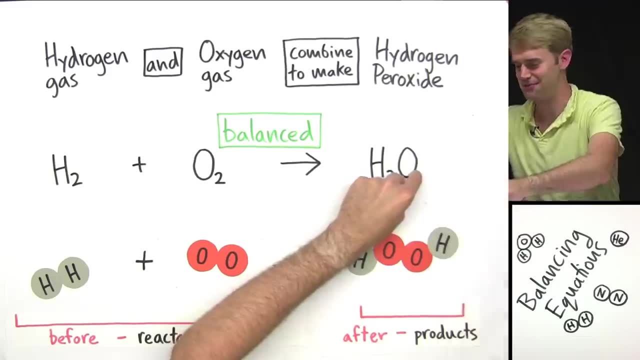 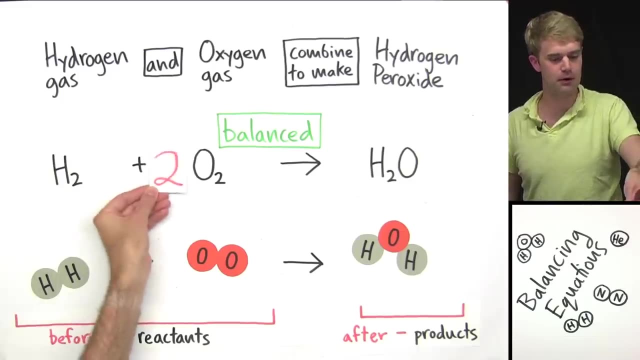 making water. It's now the equation for hydrogen gas and oxygen gas making hydrogen peroxide. You totally change the meaning of the equation if you mess around with these subscripts. So you can't do that. The subscripts have to remain the same, but you can put numbers in front of one or more. 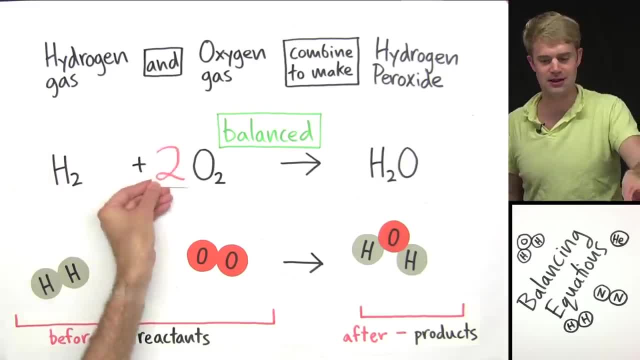 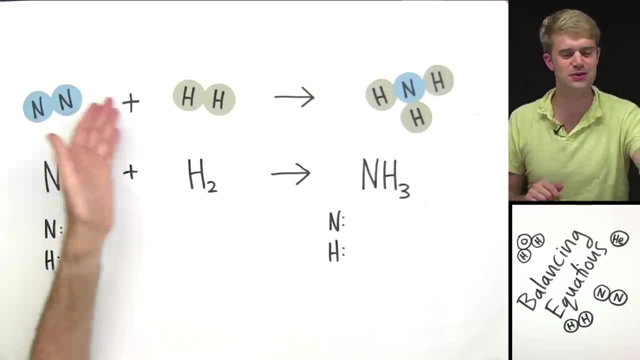 of the compounds, but the numbers always have to be in front. You can't modify any of these subscripts. When we first start off talking about balancing equations, I love to use visuals like these of the atoms and molecules so you can really see what's going on. but when you're going 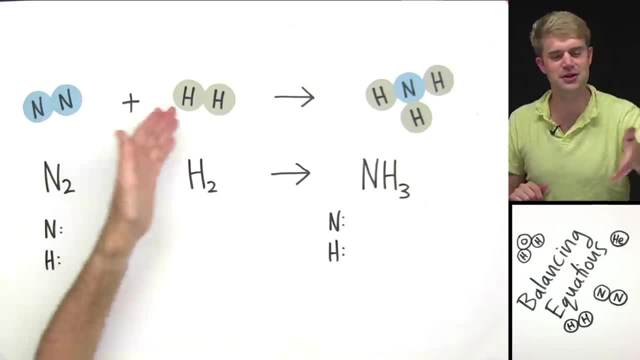 to be balancing equations on homework or on quizzes. you're not going to be using drawings like this. Instead want to be able to balance equations using charts, doing a little bit of math. so I'm going to show you one example here of how you do that. okay, so in this, 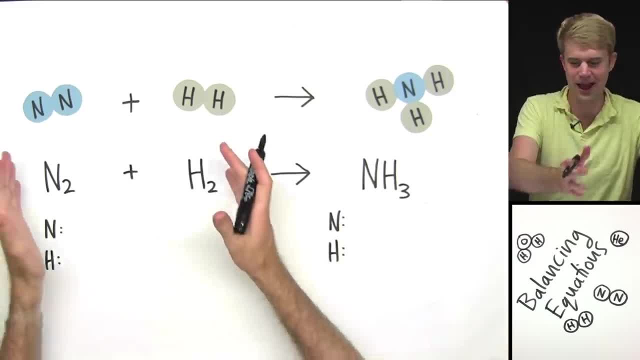 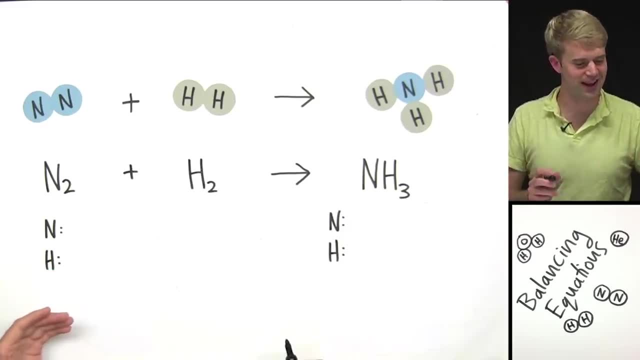 equation. we have nitrogen and hydrogen. obviously we have those on both sides. so I've made this little chart: nitrogen and hydrogen on both sides. so the first thing you want to do is you want to write in your chart how many of these atoms you have. right? so we have n2. so that means that we have two nitrogens on. 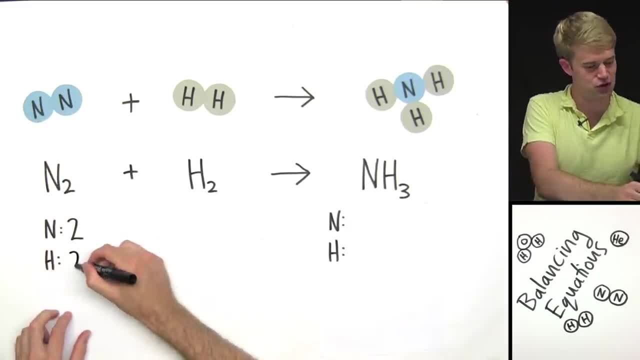 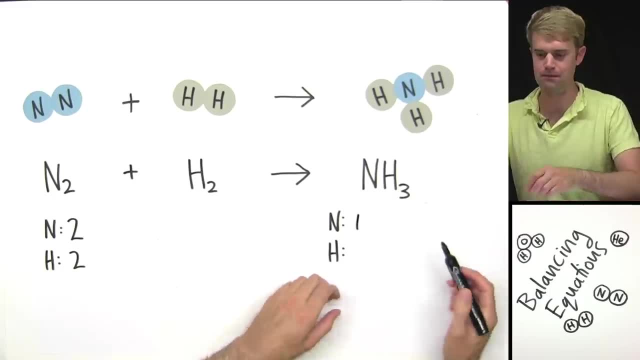 this side. you can see that from the diagram h2. we have two hydrogen atoms on this side and then we have the arrow and then over here we have n, so we have one nitrogen atom and then we have three hydrogen atoms. so to start balancing this, you want to look at where you have an imbalance of atoms, where you don't. 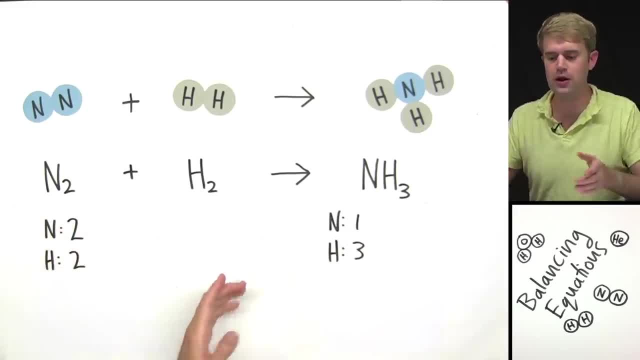 have the same number of atoms and you want to think about what you could multiply one of these compounds by. okay, so let's tell me what I have here. I have a other atom and I have a little bit of this. Let's look at nitrogen right here. 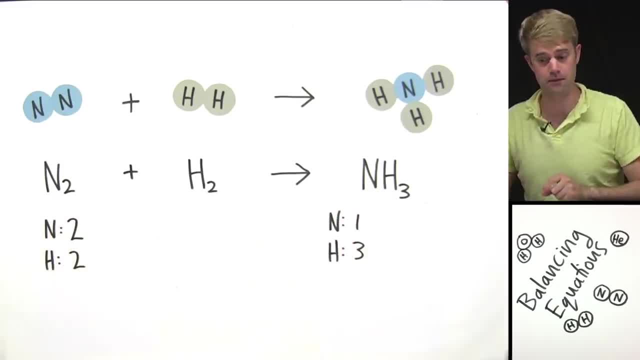 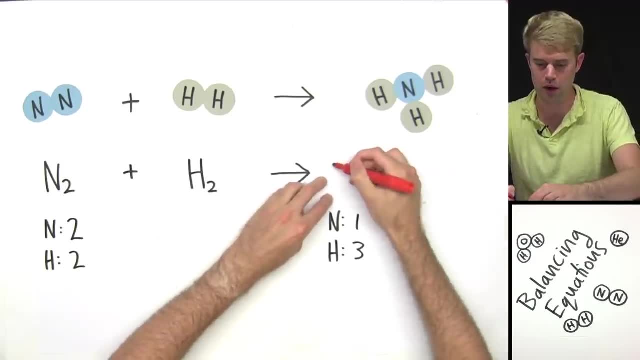 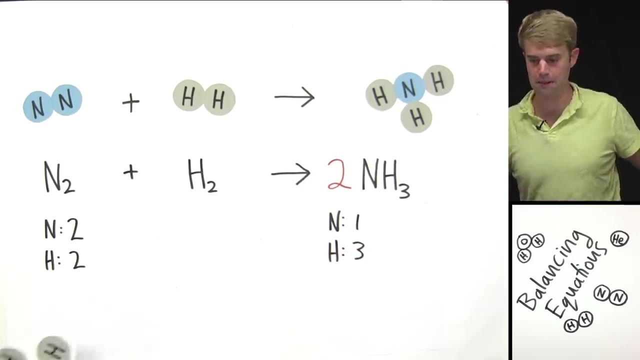 We have two nitrogens here. We only have one here. okay, So one thing that we could do to start out balancing this is we could put a 2 in front of NH3 here, So that would multiply this whole thing by 2.. 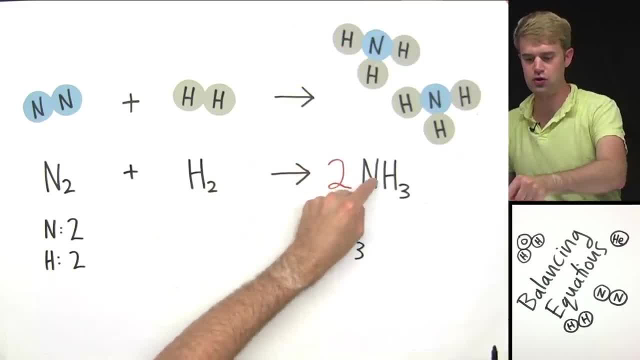 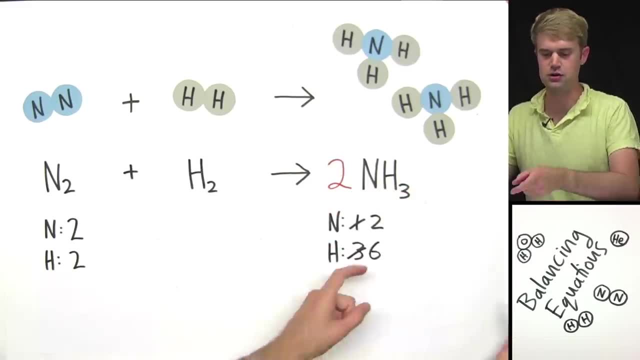 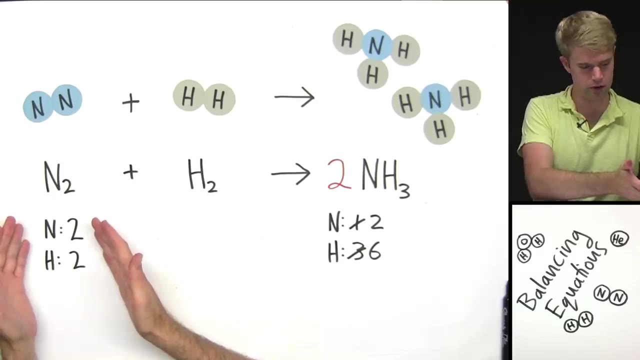 So now we'd have two of these, and that would give us two nitrogens, And now we have 2 times 3, which is going to give us 6 hydrogens. okay, So that's how we use this chart. Now, that kind of changed these numbers, so let's look at what's going on over here, okay. 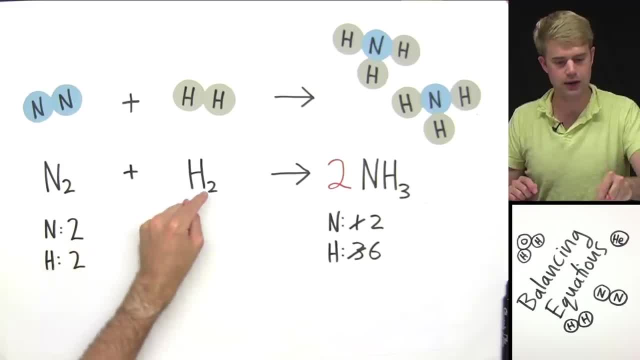 So now the nitrogens balance, but now the hydrogens don't balance. I have 6 here and I have 2 here. okay, So what could I multiply something by here to fix the hydrogens? Well, I have 2 right now. 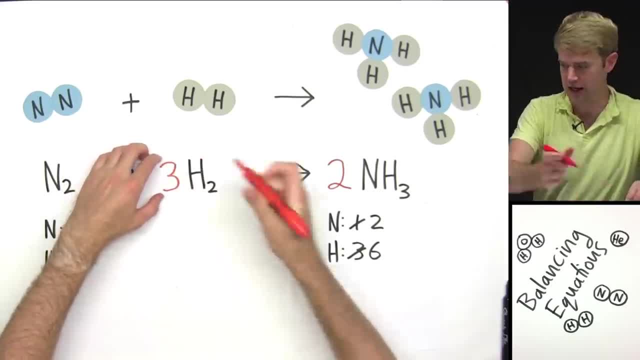 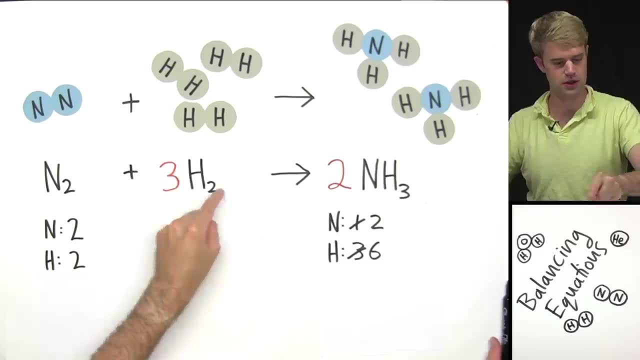 I want 6.. So I could put a 3 here, 3 in front of this. It would look like this in our visual: Now we have 2 more hydrogens and that gives us 3 times 2, 6 hydrogens here. 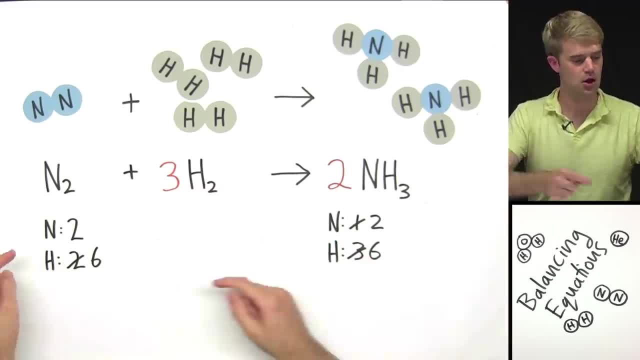 So we can keep track of these adjustments that we make using charts like this that show us how many of each atom we have on both sides. We multiply something by a number in front of it and then we change the number of atoms. So the best way to get good at this, 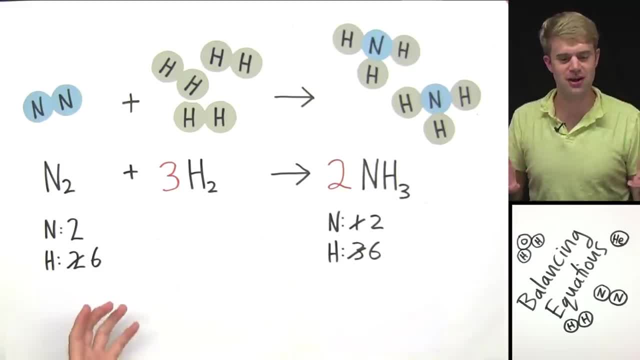 Is to just do a whole bunch of practice. Check out my video of balancing chemical equations- Practice problems. You'll do a whole bunch of examples and it will really make sense.